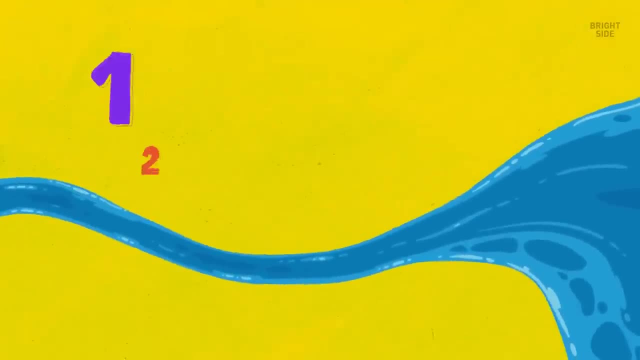 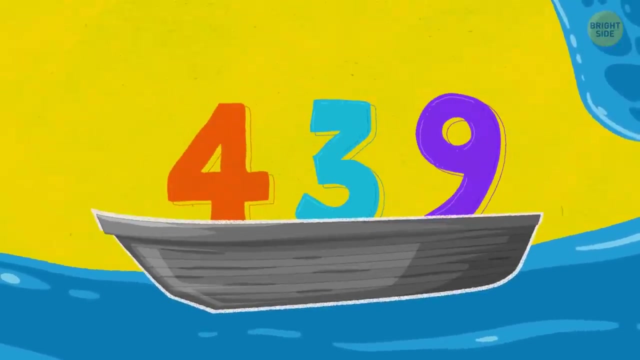 and eleven In the land of riddles. nine numbers- from one to nine- want to cross a river. There is a boat, but it can't carry more than three numbers at a time. Plus, the sum of the traveling numbers has to be a square number, and the boat can't move on its own. How many trips? 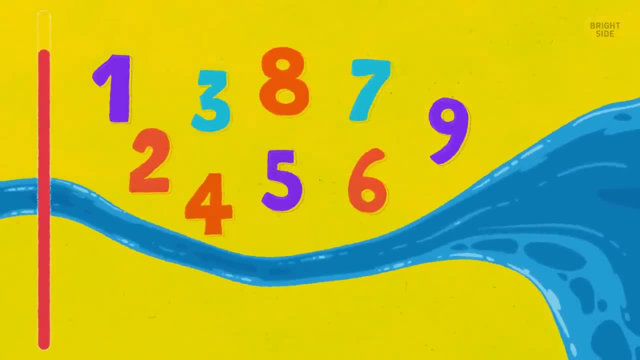 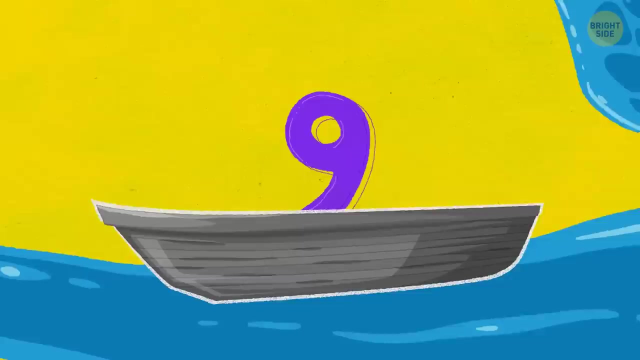 will be needed for all the numbers to cross the river. At least seven trips. Two plus five plus nine equals sixteen. then nine goes back. Three plus four plus nine equals sixteen. After that, nine returns. One plus seven plus eight equals sixteen. One goes back. And finally, one plus six plus nine equals sixteen. 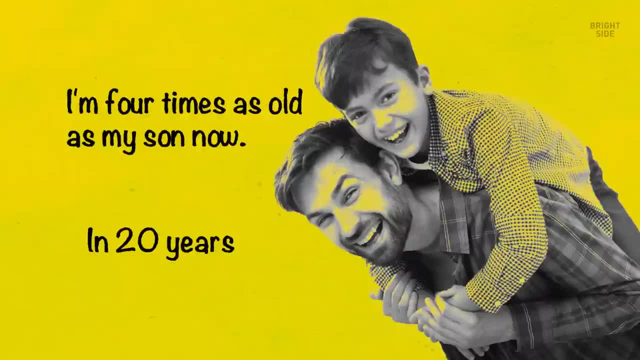 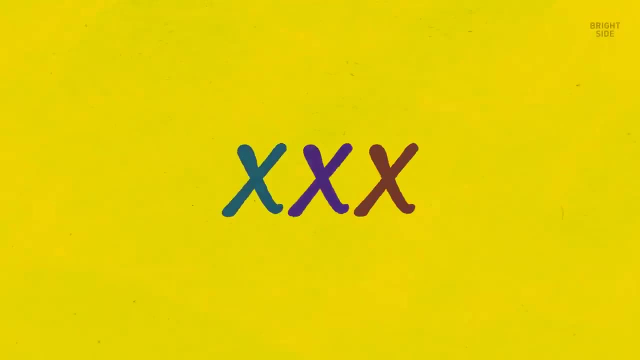 I'm forty and my son is ten. I'm a three-digit number. My second digit is four times as big as the first one And the third digit is smaller by three than the second. What number am I? I'm 141.. 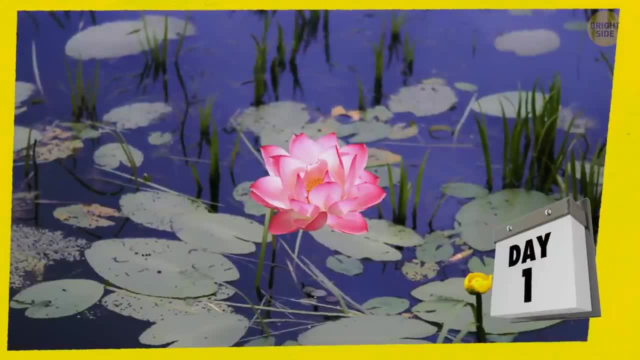 A beautiful water lily grows in the middle of a tiny pond. The flower doubles in size every day. You know that in 10 days it will cover the entire pond. The question is: in how many days will the lily cover half of the pond? 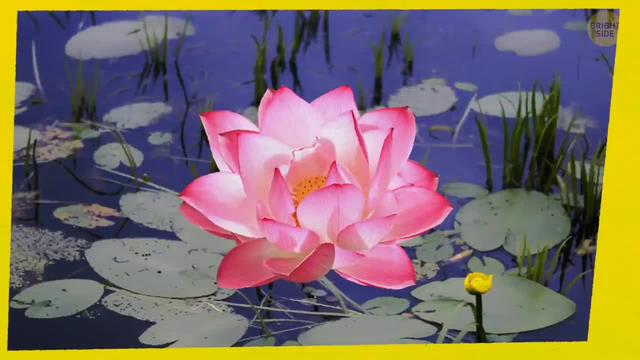 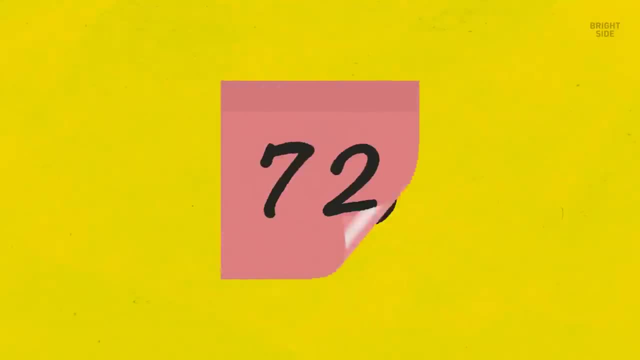 It'll happen on the 9th day. The lily doubles in size every day. It means that it'll cover half of the pond one day before it covers the entire pond. How can you turn 98 into 72 by using just one letter? 1., 2., 3., 4., 5., 6., 7., 8., 9., 10., 11., 12., 13., 14., 15., 16., 17.. 18., 19., 20., 21., 22., 23., 24., 25., 26., 27., 28., 29., 30., 31., 31., 32., 33.. 34., 35., 36., 37., 37., 38., 38., 39., 39., 40., 41., 42., 42., 43., 44., 44., 43.. 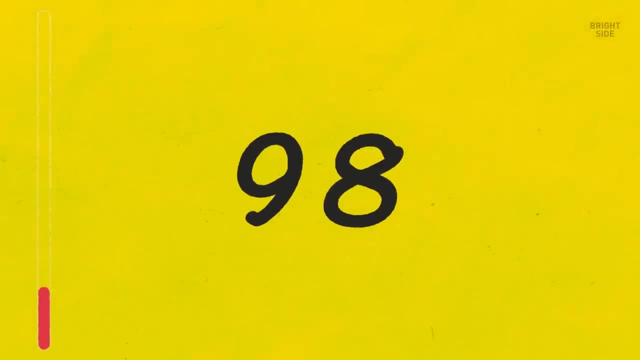 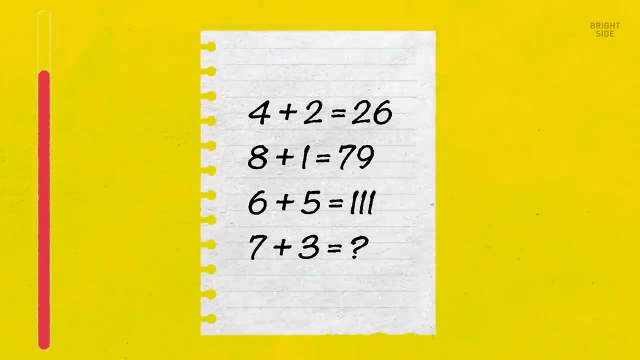 44., 45., 46., 47., 47., 49., 48., 58., 51., 52., 52.. 4 plus 2 equals 26,, since 4 minus 2 equals sign 2, and 4 plus 2 equals 6,, 8 minus 1 equals. 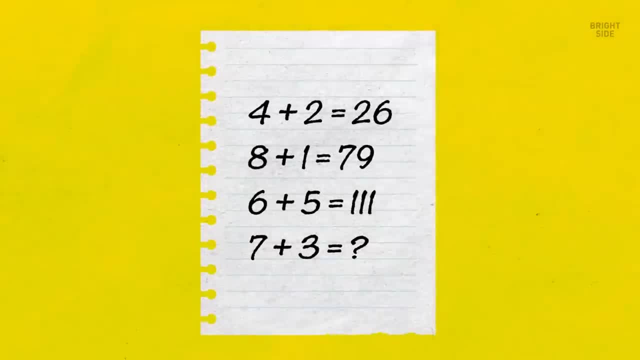 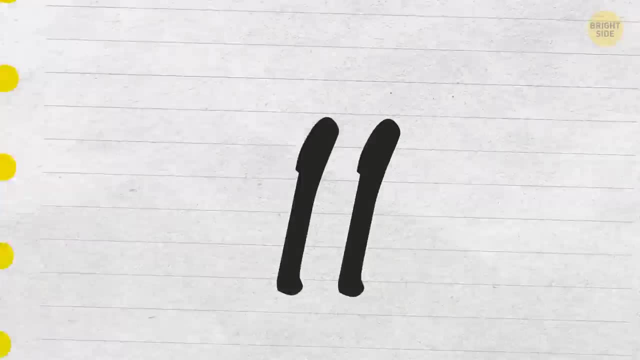 sign 7, and 8 plus 1 equals 9, and so on. 7 minus 3 equals sign 4, and 7 plus 3 equals 10.. It means the answer will be 410.. Which number's missing? 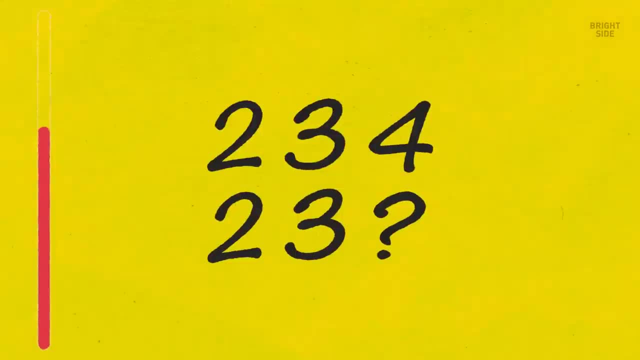 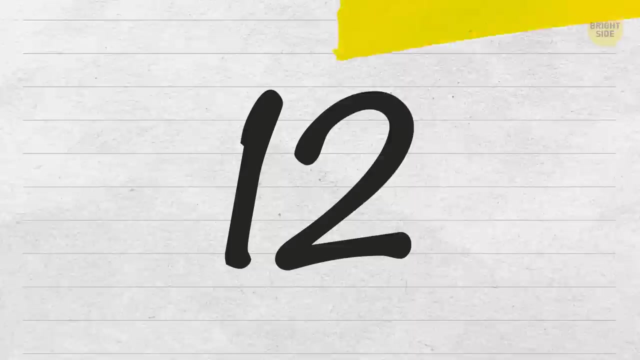 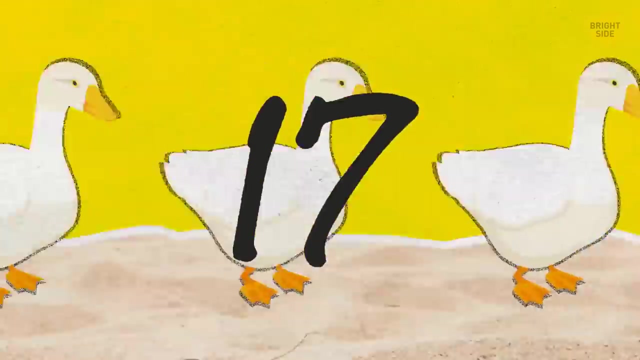 Nope, it's not 4.. The missing number is 5.. You need to get subsequent 234 and 235.. The geese were going to the watering hole in a single file, one after another. One goose looked ahead and saw that there were 17 birds in front of it. 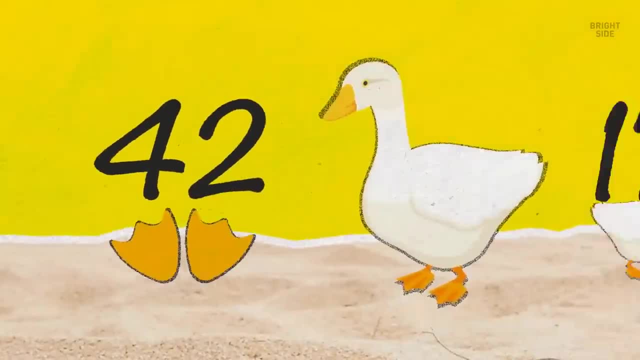 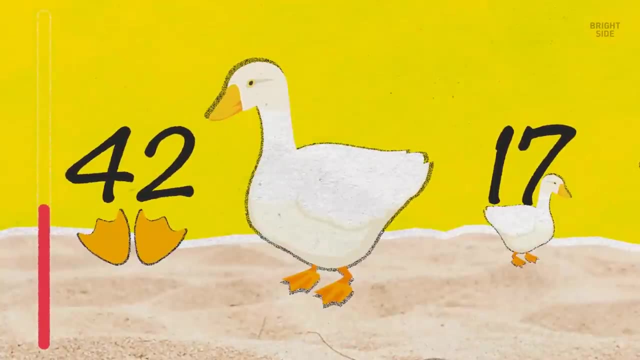 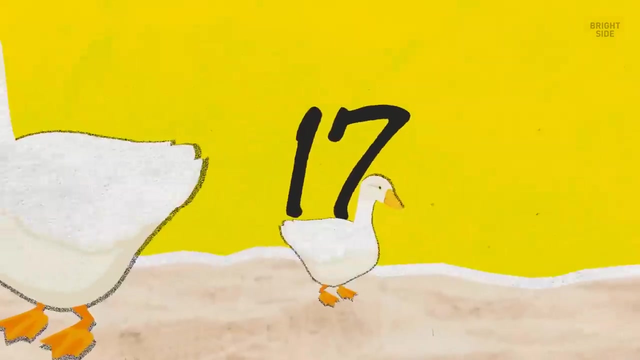 It looked back, Forty-two paws were following him. How many geese were there? Answer: 39.. Seventeen in front, 21 behind and the goose who counted, A hen and a half, lay an egg and a half in a day and a half. 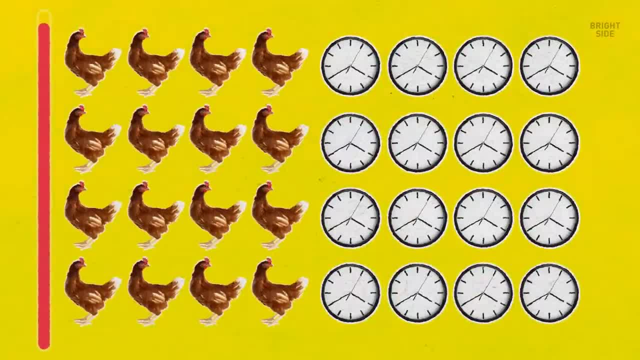 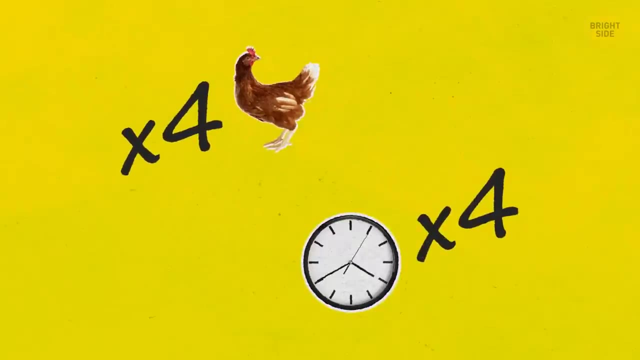 How many eggs will half a dozen hens lay in half a dozen days? Twenty-four. If there are four times more hens and they have four times more days, they will lay sixteen times more eggs. Sixteen x one point five equals, sign twenty-four eggs. 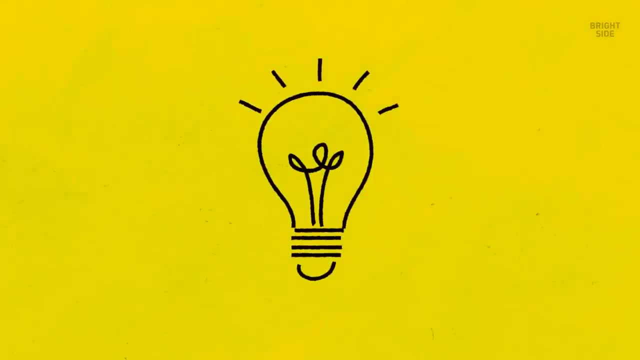 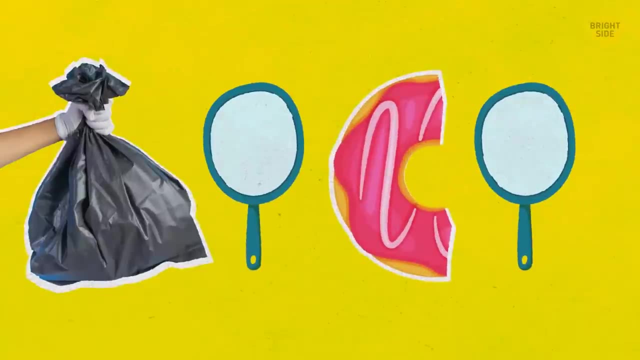 I'll give you three clues, and your task is to find a four-digit number. Its first digit is useless, The second and fourth digits are mirror images of each other, and the third digit is half the second. What is the number? Twenty-four? 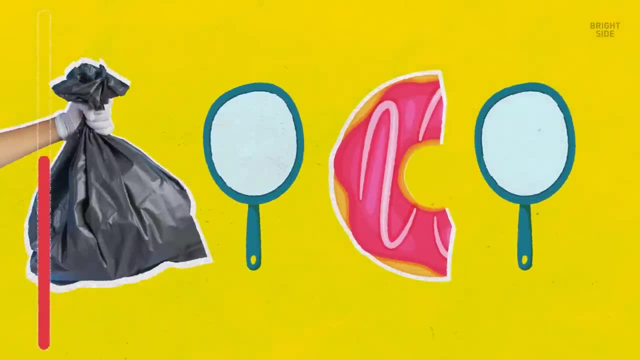 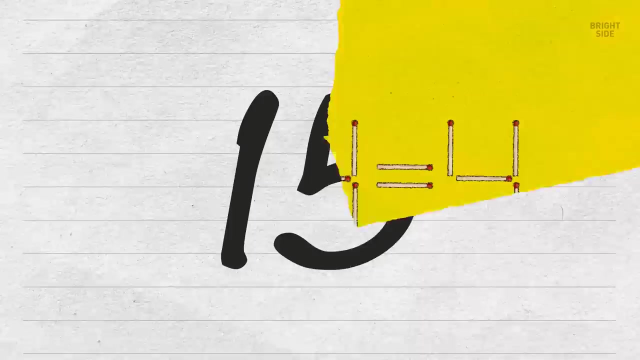 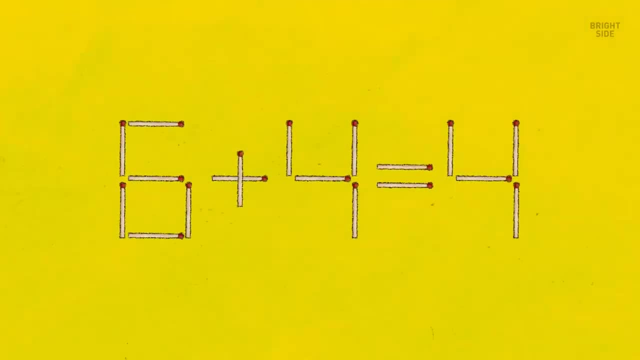 You have an equation made from matchsticks. Six plus four equals four. Move just one matchstick. to make it true Twenty-four, You need to take one matchstick from the plus sign and add it to 6 so that it makes 8.. 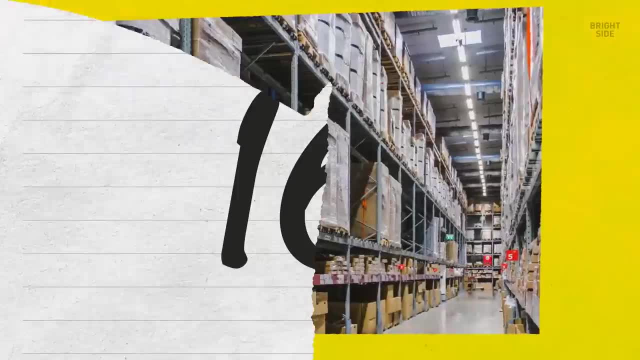 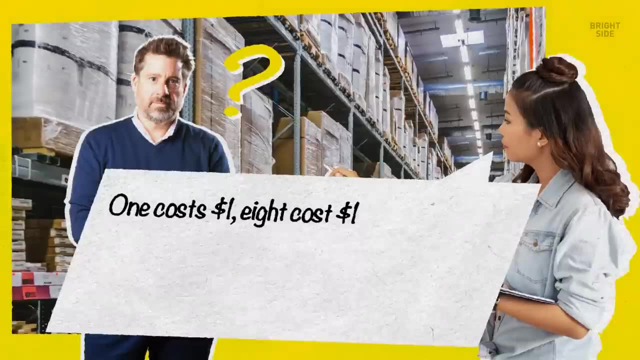 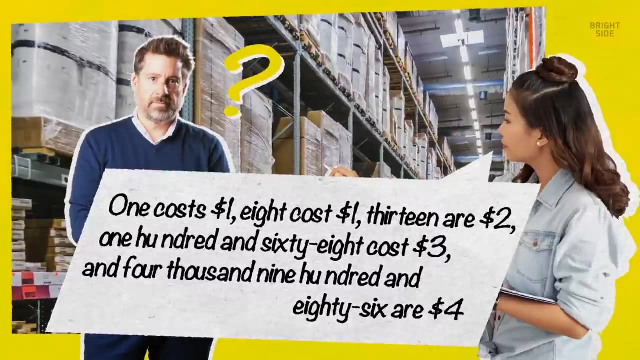 Then you'll have 8 minus 4 equals 4.. A man walked into a hardware store and asked the price of one item. The seller replied: 1 costs $1,, 8 costs $1,, 13 are $2,, 168 cost $3, and 4,986 are $4. 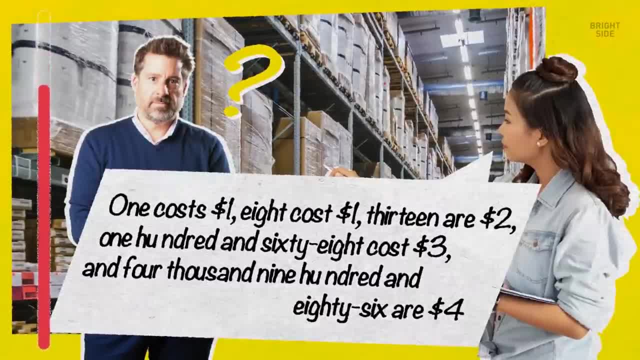 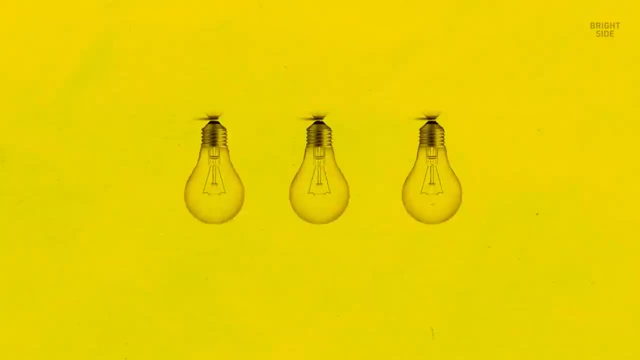 What did the man want to buy? He was interested in door numbers. Imagine standing in front of a closed room that has three light bulbs. All of them are currently turned off. There are three switches in front of you that are responsible for the light bulbs. 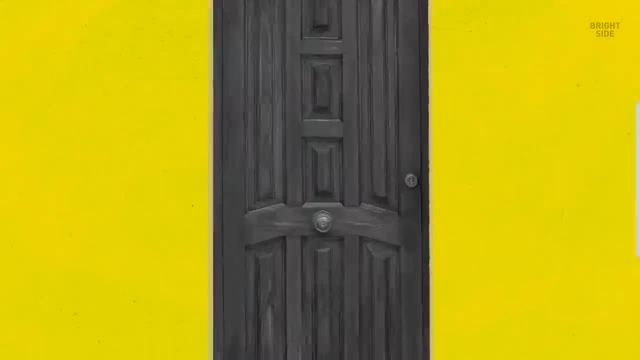 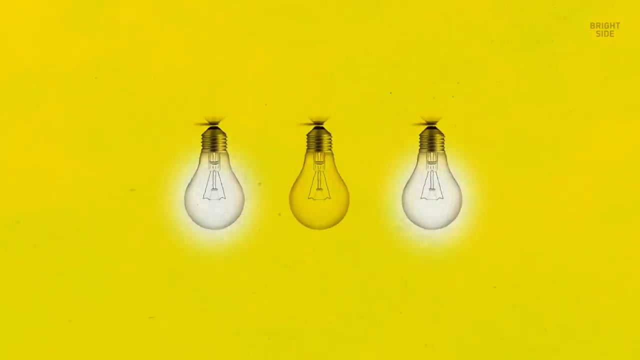 You can turn the lights on and off as many times as you like, but you can enter the room only once. Also, you do not know which switch is connected to which light bulb. After entering the room, you can do whatever you want with the light bulbs, but you can't. 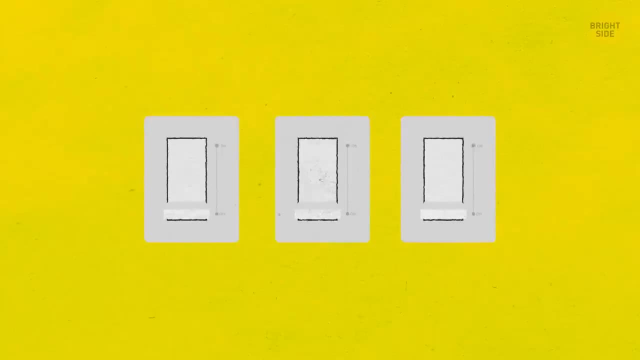 go back to the switches. You need to figure out which switch is responsible for which light bulb. Turn on the first switch and leave it on for some time. Do not touch the second switch at all, but turn on the third switch, Wait for a few minutes and then turn it off again. 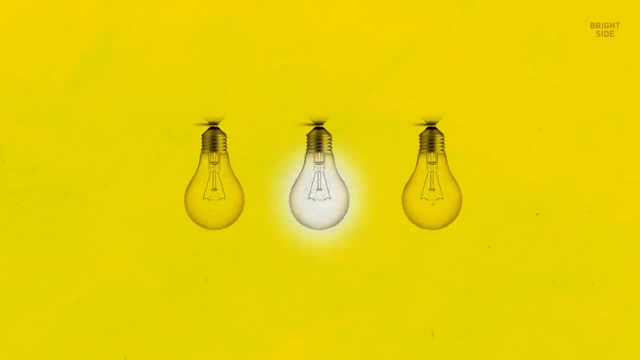 Now, when you enter the room, you will find one brightly lit light bulb, One light bulb that is turned off and, at the same time, cold to the touch, and one that is also turned off but warm to the touch. Based on this, you will be able to understand which switch is connected to which light bulb. 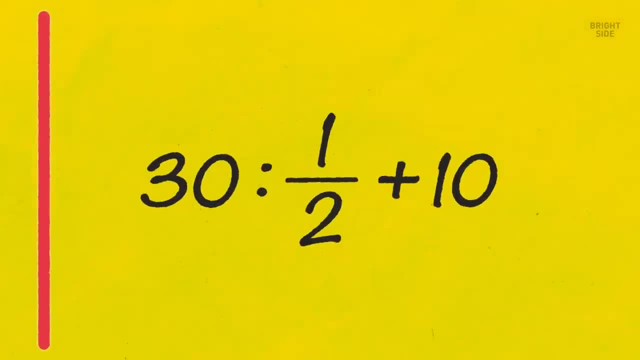 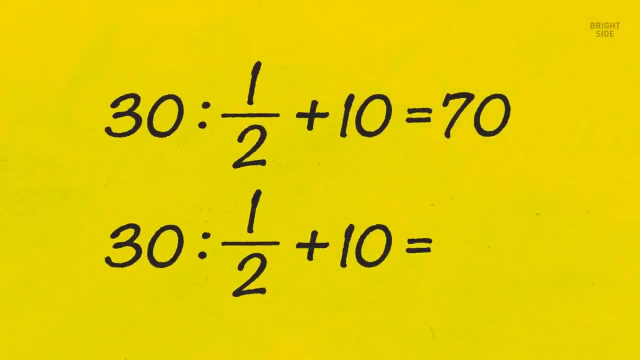 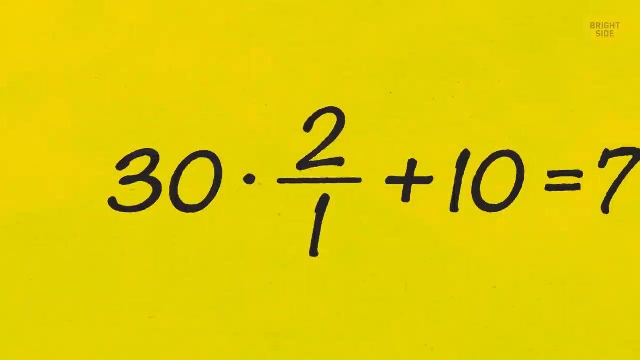 Divide 30 by 1 half and add 10.. What will be the result? It's 70.. Most people count like this: 30 halves plus 10 equals sign 25.. But when you divide some number by a fraction, you actually have to multiply it by the inverted fraction. So 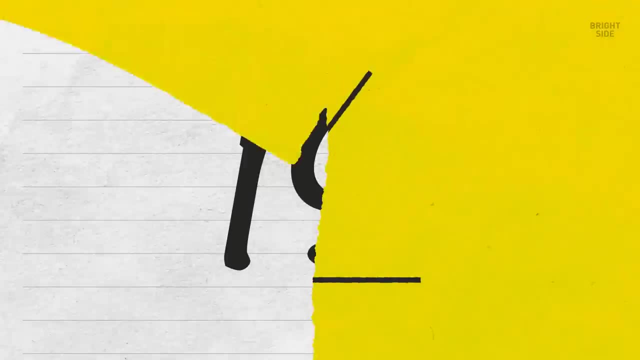 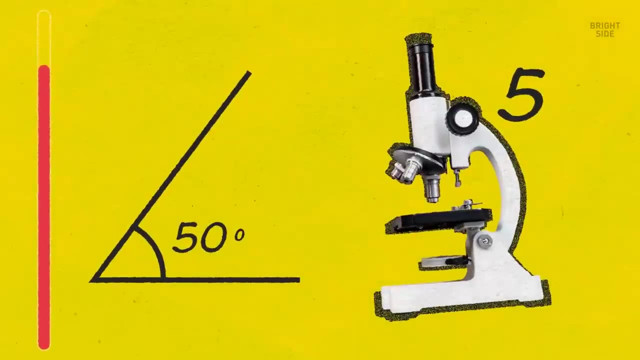 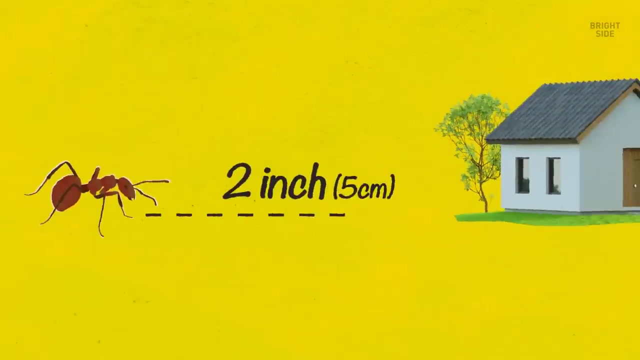 30 by 2 plus 10 equals 70.. How much will a 50 degrees angle measure? if you look at it through a microscope that magnifies objects five times, The angle won't change, It'll still be 50 degrees. An ant is two inches away from its home With every next step. 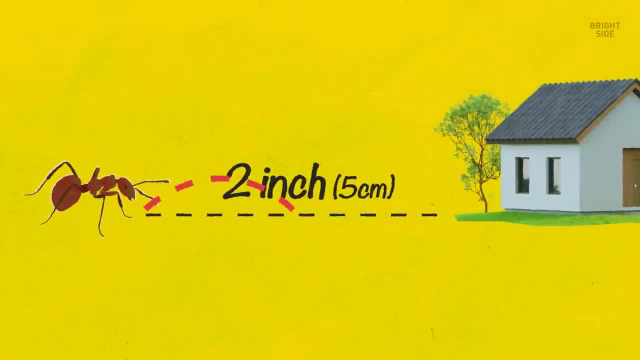 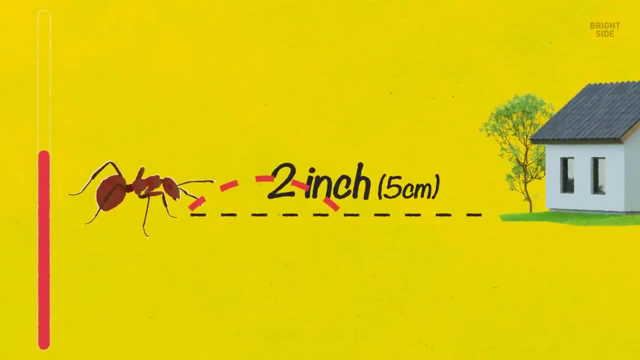 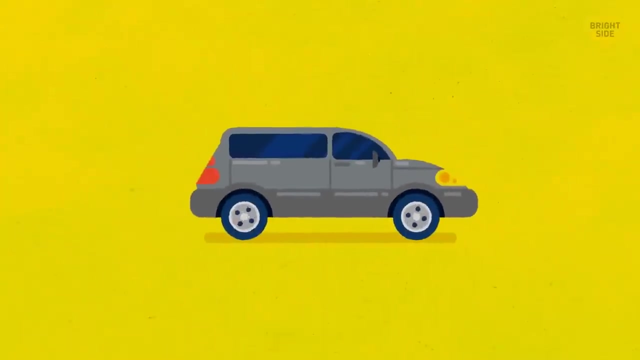 the insect covers half the distance to the entrance. How many steps will it take for the insect to reach its destination? The ant will never reach the door because every time it'll travel only half the distance. Three friends went on a road trip. They rented a triple room in a hotel for a night. When 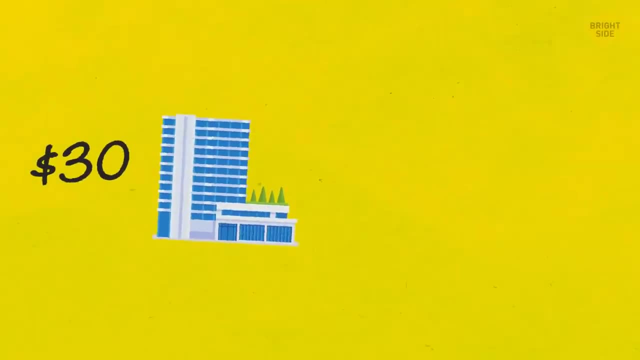 they got to the hotel they paid $30 and went up to their room. The porter brought their bags up and gave them $5 back because the hotel was running a weeknight special. There are items they need to take with them. We can share a few of them with you. 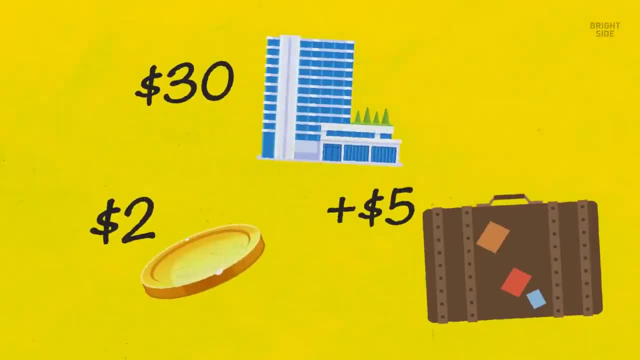 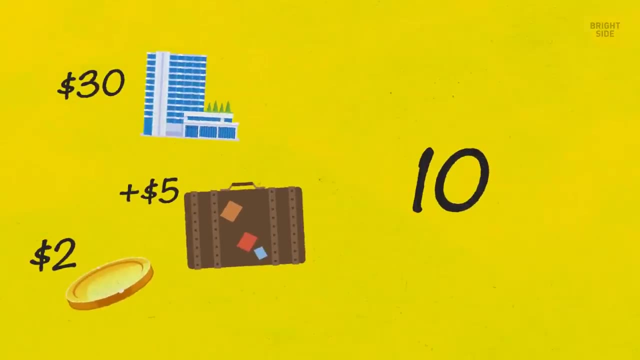 Until we meet again next time. The friends each took $1 and gave the porter $2 as a tip. Later they decided to write down their expenses for the weekend and found out they had a problem. They each paid $10 for the room and got $1 back. 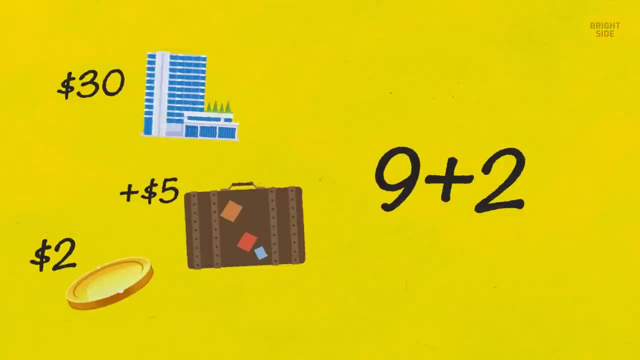 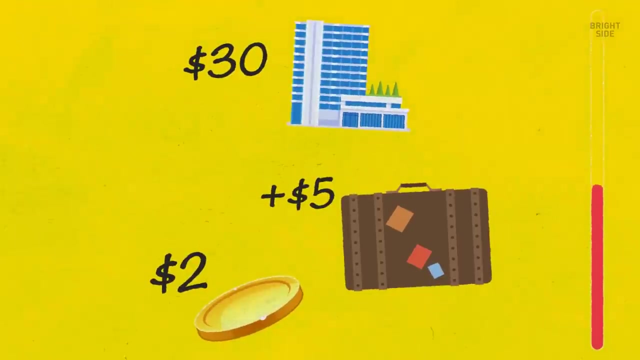 which made their contributions $9. Then they gave the porter a $2 tip, but 9 times 3 is 27,, and 27 plus 2 is $29.. Where did the extra dollar go? I admit this riddle might seem a bit twisty. 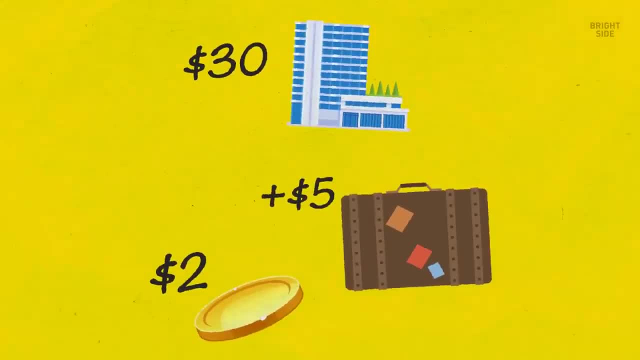 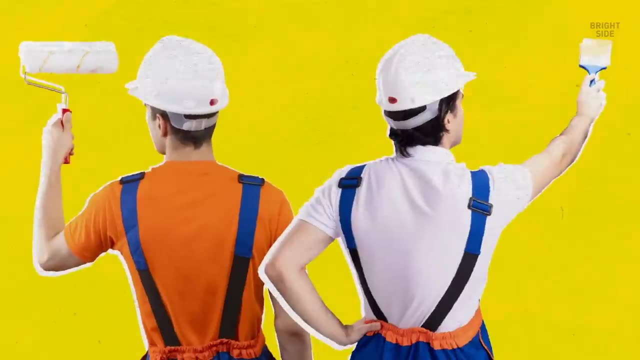 but what it boils down to is that the three friends' math is wrong. Having finished all the work, two painters went home. On the way they met two other painters. they knew quite well How can the first two painters shake hands with the other two painters. 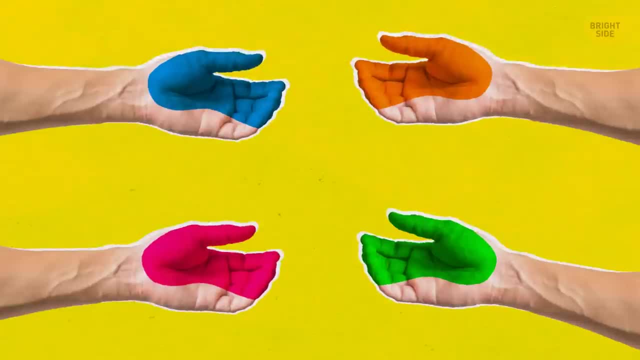 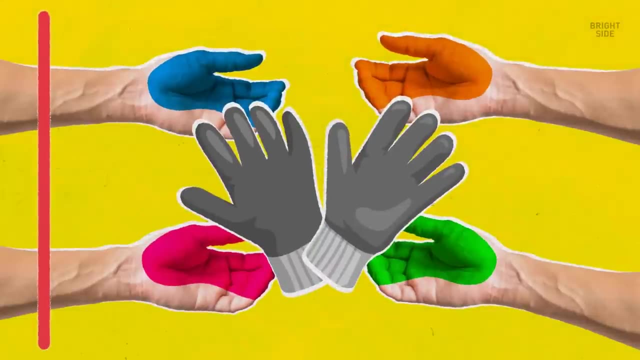 and not get their hands even dirtier, given the fact that their hands are all covered in different paints. Keep in mind that, luckily, all the painters have two gloves that can be passed to others. Let's give our painters some names. Let the first two be A and B. 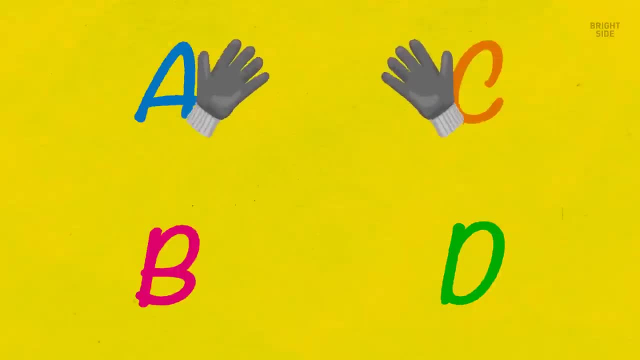 then the second two will be C and D. Painters A and C put on the gloves and greet each other. Now these gloves are stained on one side with the paints they worked with, but the other side of the gloves is still clean. Painter A and C are still clean. 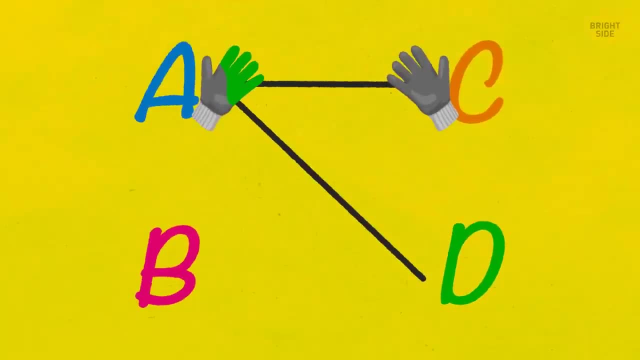 Painter A rearranges his glove and greets D. The glove gets completely dirty, But A can turn the glove inside out and give it to D. painters C and B repeat this process. Lastly, B and D greet each other using the gloves turned inside out. 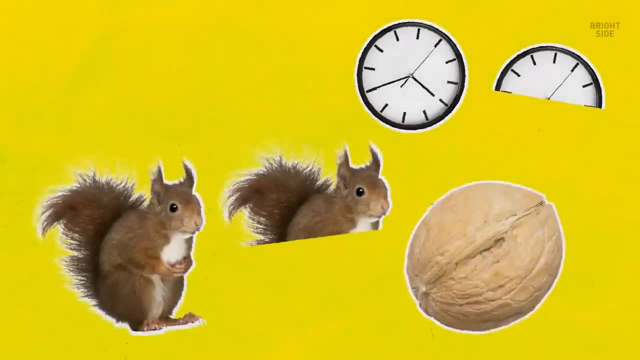 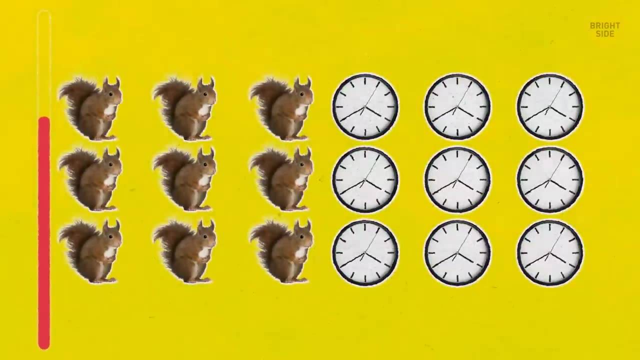 In 1.5 minutes one and a half squirrels gnaw 1.5 nuts. How many nuts can nine squirrels chew in nine minutes? I don't know about you, but my first impulse was to answer nine. But it can't be that simple right. 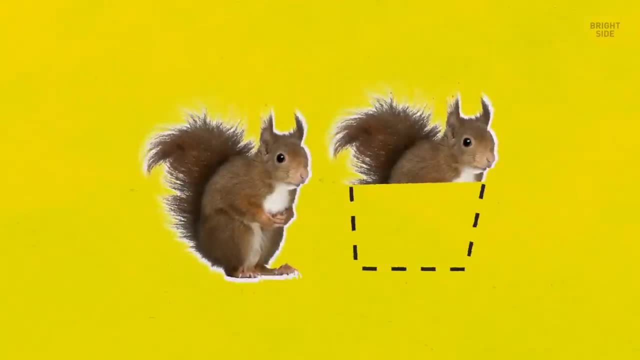 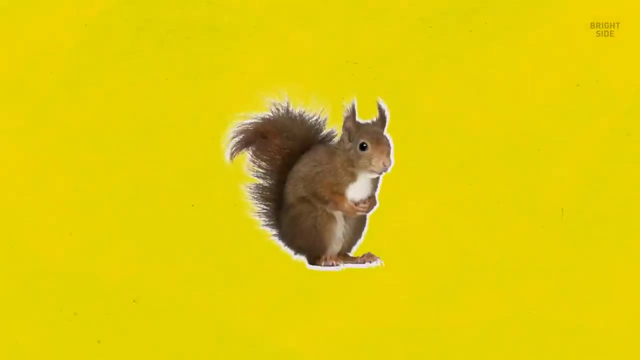 The key point lies in the conditions of the problem, where one and a half squirrels appear. To find the right answer, let's get rid of half of the poor animal and start working with whole numbers. Let's determine how many nuts one squirrel can chew in 1.5 minutes. 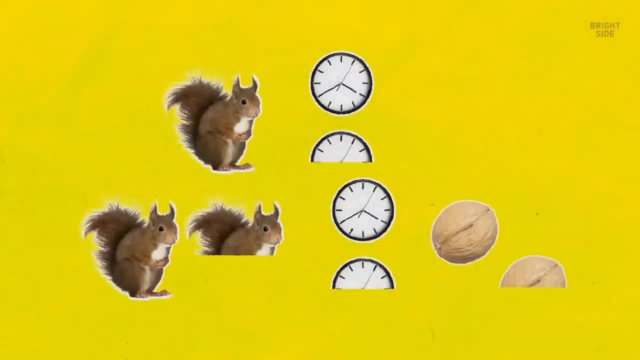 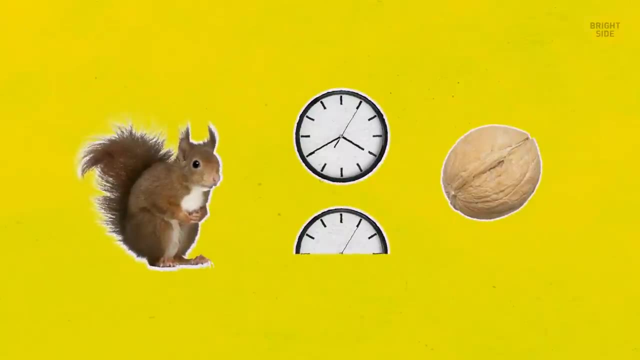 If one and a half squirrels gnaw one and a half nuts in one and a half minutes, then one squirrel in the same minute and a half gnaws one nut. The next step is to figure out how many nuts the squirrel will chew if you give it nine minutes. 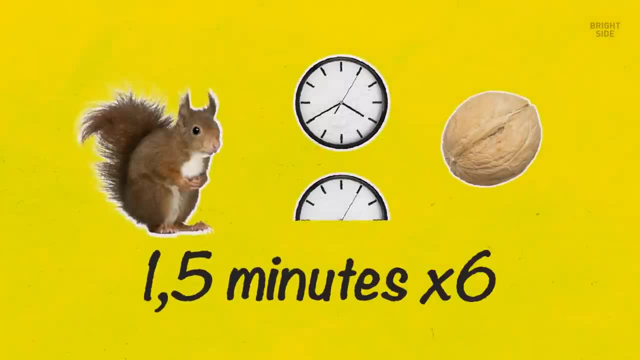 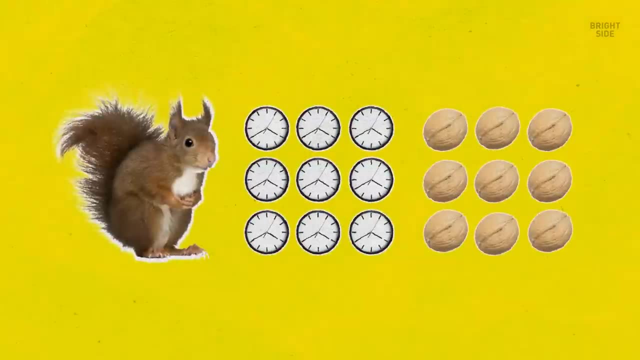 To do it, we need to multiply 1.5 minutes by six. It means that the number of eaten nuts also needs to be multiplied by six. So one squirrel chews six nuts in nine minutes. Now all we need to do is to increase the number of squirrels to nine. 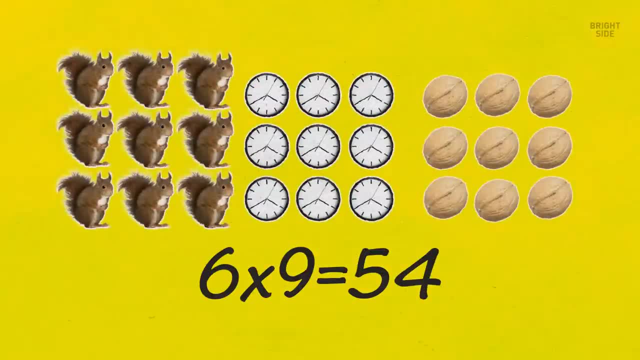 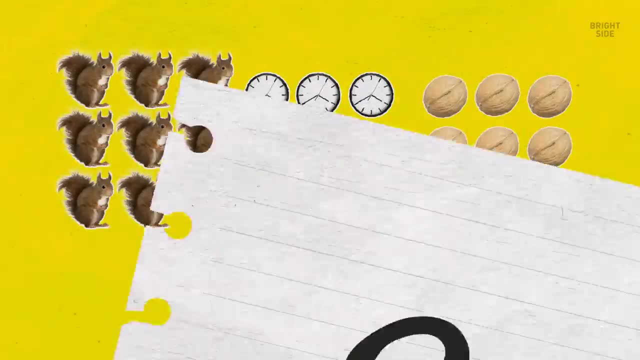 and calculate how many nuts they will eat during the same nine minutes, And we get the answer: Nine squirrels will chew 54 nuts in nine minutes. No magic, simple arithmetic. In this image you can see some yummy rolls. These two rolls, orange and black, cost $7. 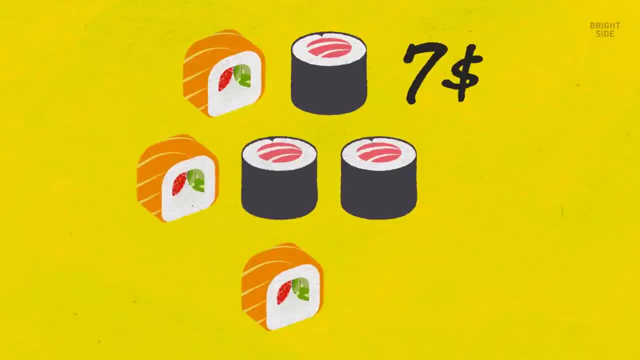 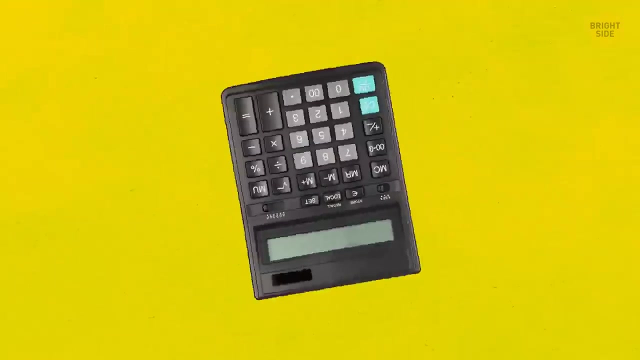 There are three rolls on the middle shelf, two black and one orange, And together they cost $12.. There is one orange roll on the third shelf. How much does it cost? $12.. The price is $2.. Now don't take the following riddles too seriously. 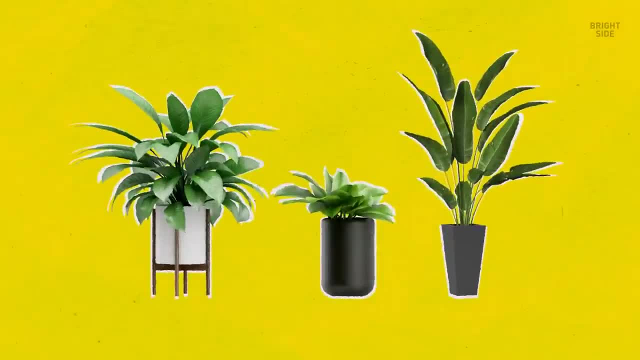 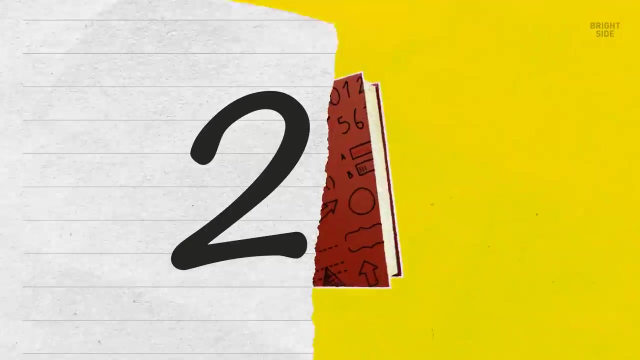 Try to think outside the box. What usually happens with plants in math classrooms? They grow square roots. What did one math book tell another? The answer is a square root. What did one math book tell another? The answer is a square root. 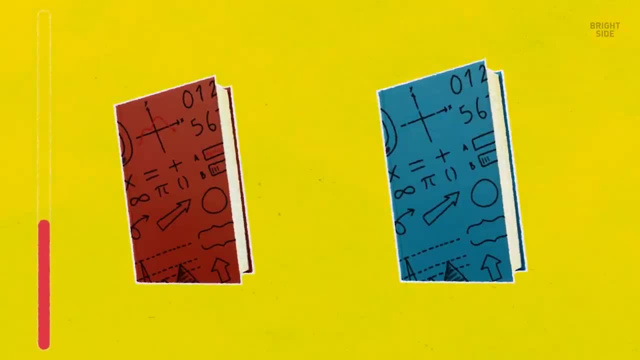 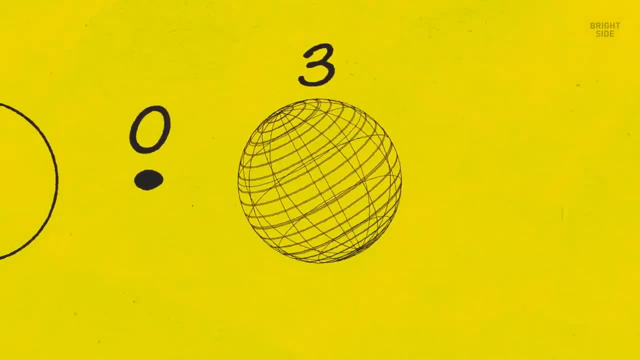 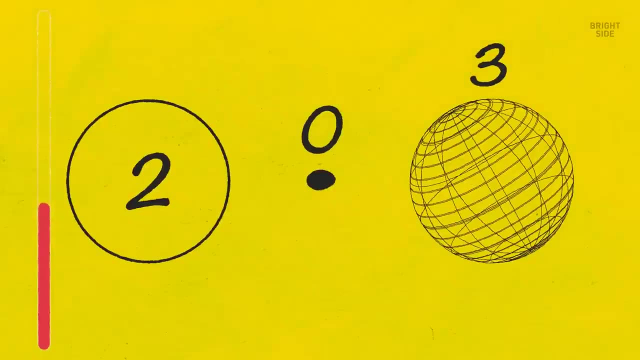 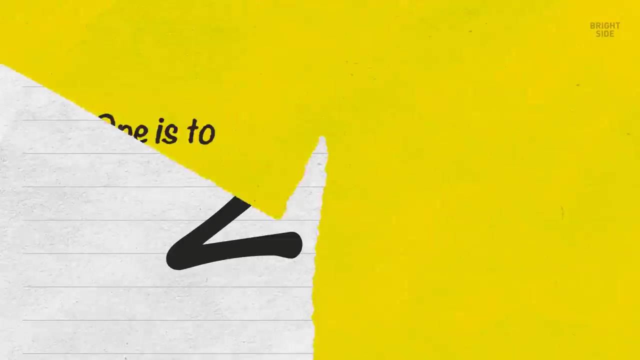 A circle has two, a point has zero and a sphere has three. What am I talking about? Dimensions? One is to three, as three is to five And five is to four, And four is the magic number. Can you figure out the pattern? 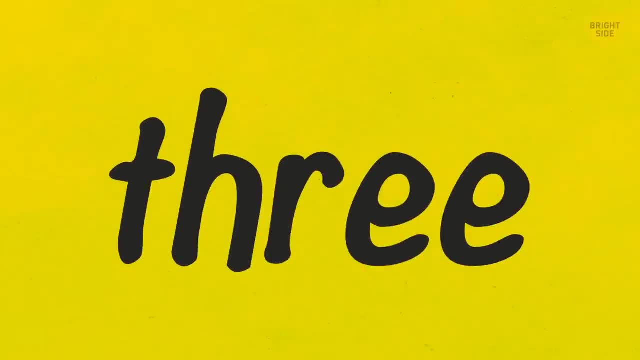 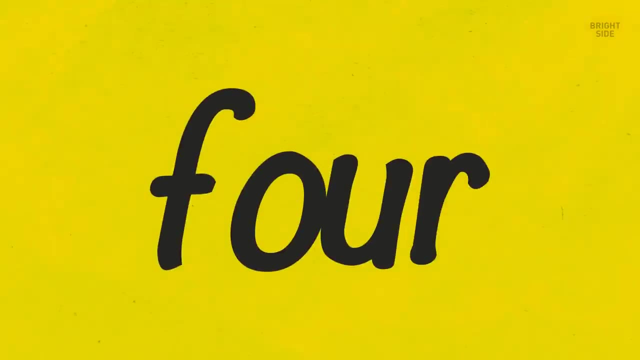 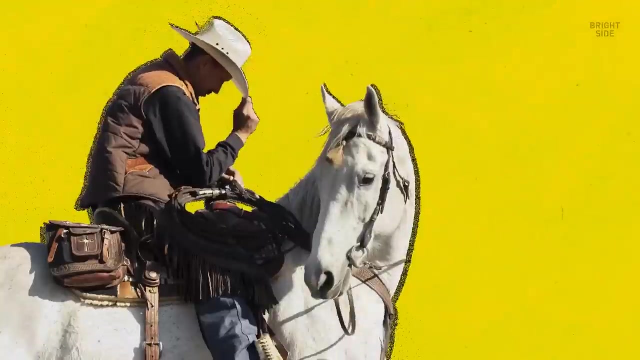 The word one has three letters, the word three has five and the word five Consists of four letters. but the word four has four letters in it and whatever number you try, eventually you'll come back to four. That's why it's a magic number. Horses and people are gathered in a stable. You know that in total there are 72 legs and 22 heads. 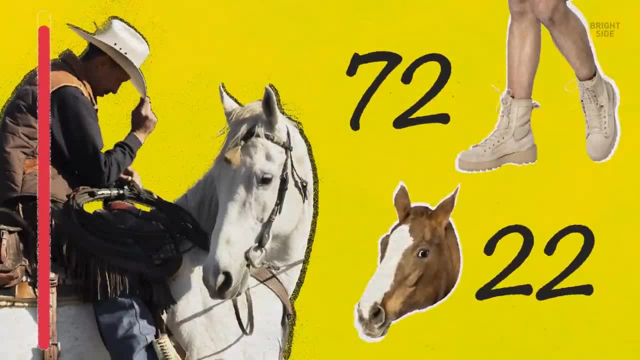 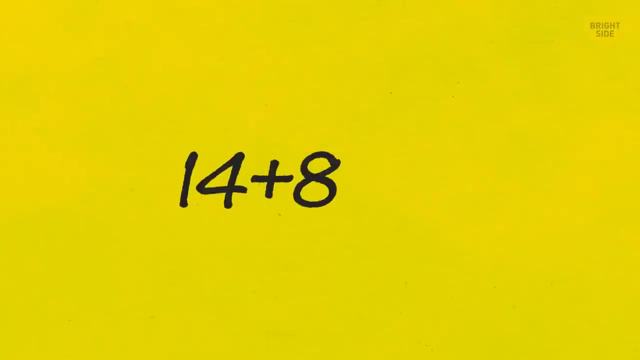 How many horses and how many people are there in the stable? There are 14 horses and 8 people. 14 plus 8 equals 22 heads. 14 x 4 plus 8 x 2 equals sign 72 legs. That's it for today. 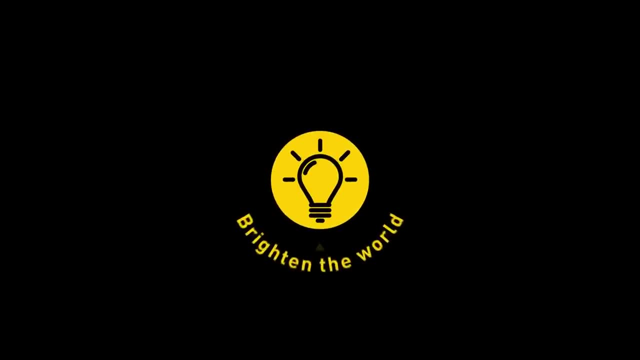 So, hey, If you pacified your curiosity, then give the video a like and share it with your friends. or if you want more, just click On these videos and stay on the bright side.